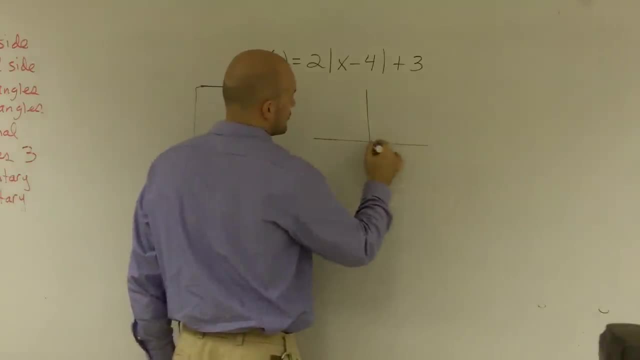 that a regular graph, without any alterations, f of x equals f of x. So f of x equals absolute value of x is right there, right, Not shifted up and down. It has a vertex at 0, 0. And it goes up, has two points that we know, which is 1 comma 1 and negative 1 comma 1,. 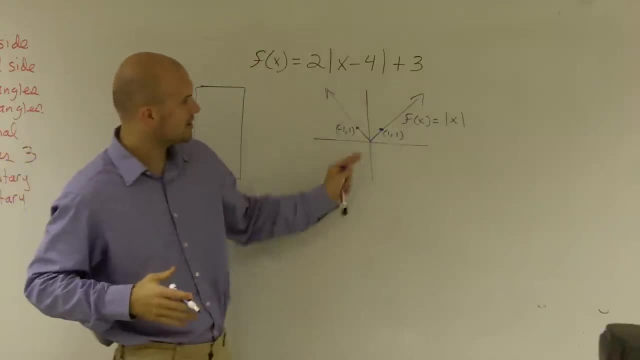 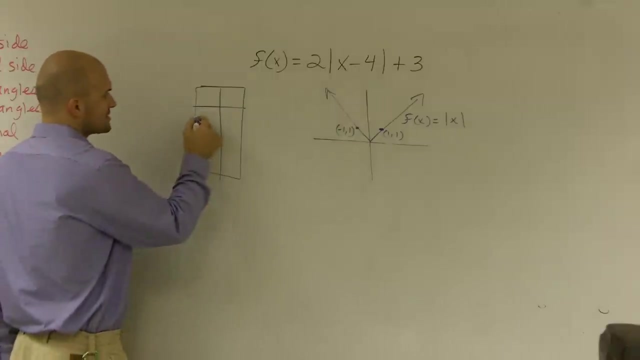 right, We actually know the rest of them. The slopes are 1 over 1, going to the infinity and negative infinity. Well, let's say I was going to go and pick two points, right, And let's say I just picked the points negative: 1, 0, and 1, all right, 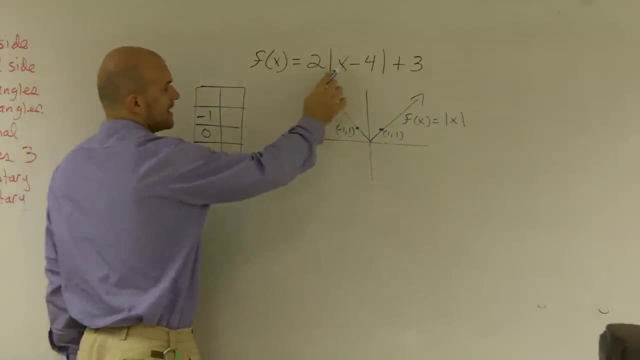 And let's say I wanted to graph this equation. Well, if I did negative 1,, 0, and 1,, I would get negative 1,. negative 1 times negative 4 is a negative 5.. Negative 5, absolute value is 5.. 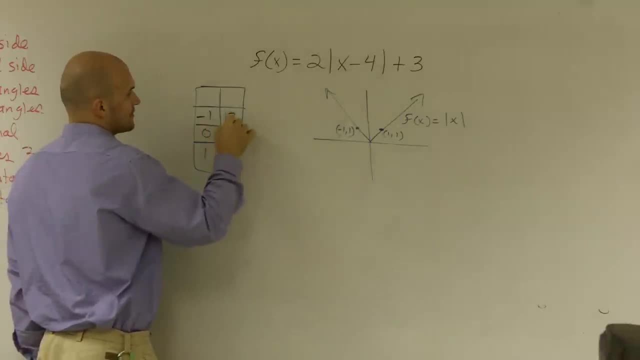 5 times 2 is 10, plus 3 is 13.. 0, 0 minus 4 is a negative 4.. Absolute value of negative 4 is 4.. 4 times 2 is 8.. 8 plus 3 is 11.. 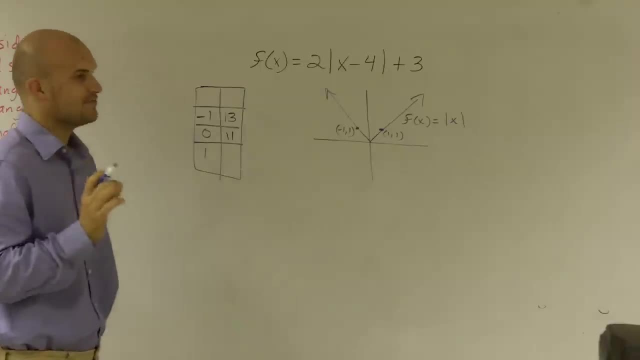 1, 1 minus 4 is negative 3.. Absolute value of negative 3 is 3.. 3 times 2 is 6.. 6 plus 3 is 9.. So if I was to graph this equation, or if I was to graph this, 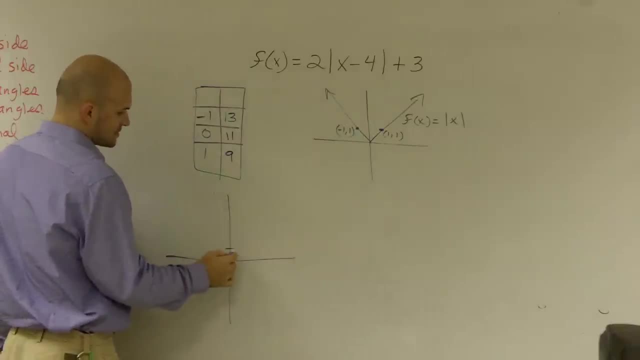 I come up with a problem because negative 1 goes up to 13. Let's see 1,, 2,, 3,, 4,, 5,, 6,, 7,, 8,, 9,, 10,, 11.. 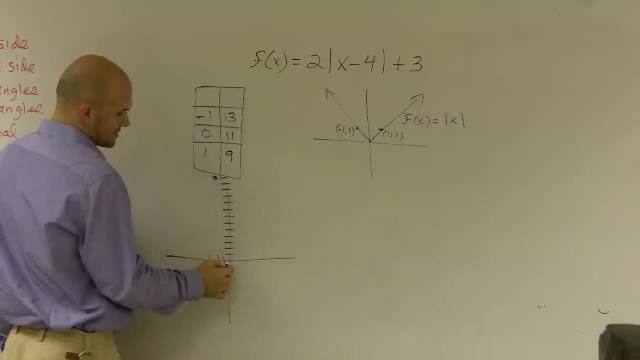 So negative 1 goes up to negative 13.. 0 goes to 11. And 1 goes to 9.. Well, that's a straight line, ladies and gentlemen. Right, So I got a big issue with this one because it's giving me a straight line. 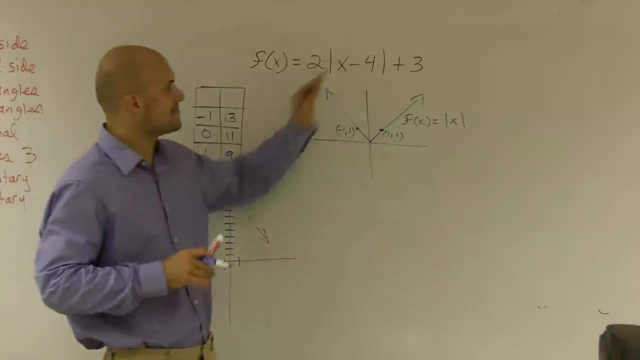 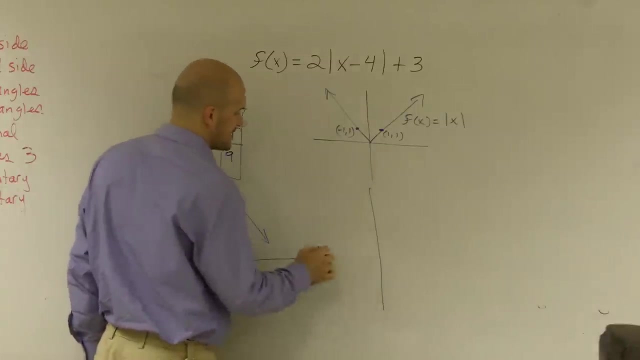 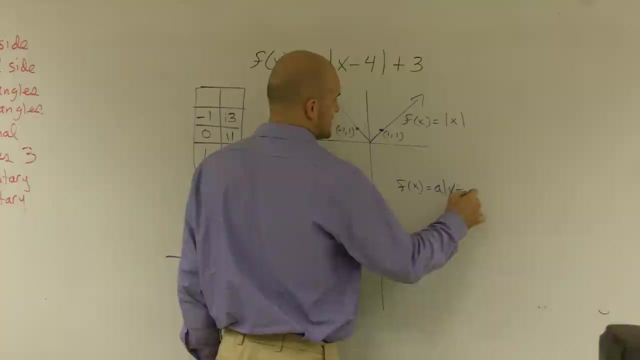 It doesn't look anything like a v. So when you see an absolute value function, a very easy way to graph this is to first find our vertex. So to do that we need to know our transformations, And the transformations is: f of x equals a times absolute value. 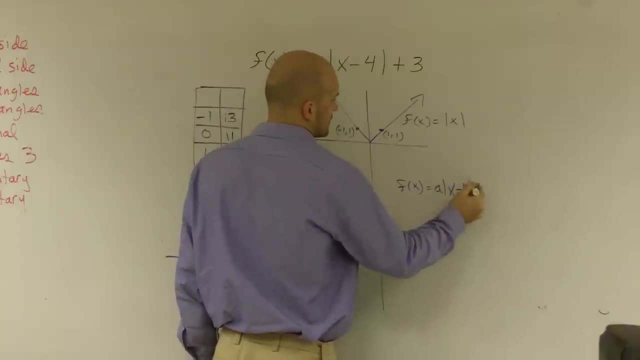 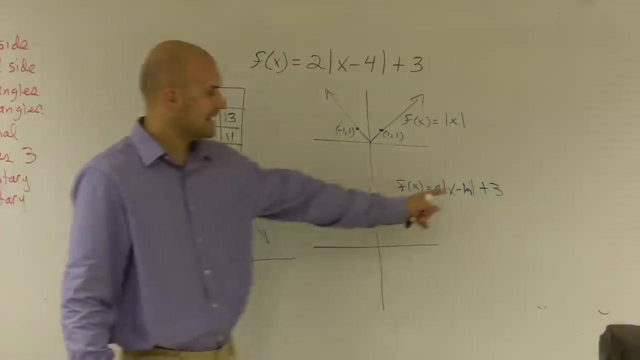 of x minus h, x minus h plus 3.. Where my h is going to tell me where to shift left or right and my k is going to tell me where to shift up or down. So if originally, without any alterations, I have my vertexes at 0, 0,, if I go ahead and alter this now, 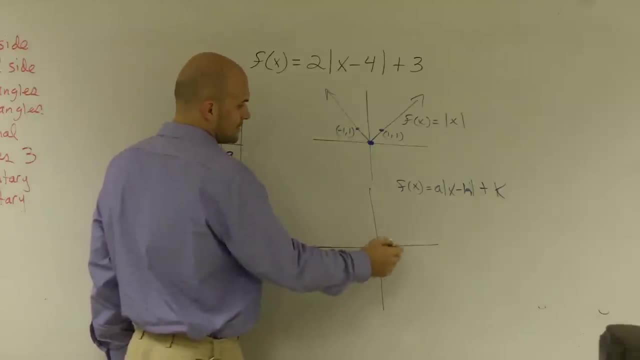 I'm going to shift 4 units to the right: 1,, 2,, 3, 4.. Right Negative h tells me to shift 4 units to the right, And then my 3 tells me to shift 3 units up. 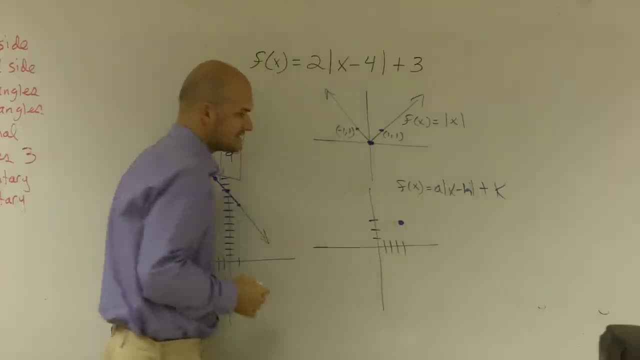 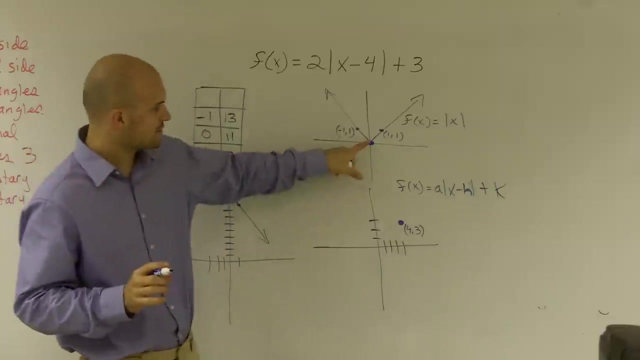 1,, 2, 3.. So therefore, now my new vertex is at 4 comma 3.. All right, So you want to find your new vertex. So pretty much what I did was I just shifted this point to over here. 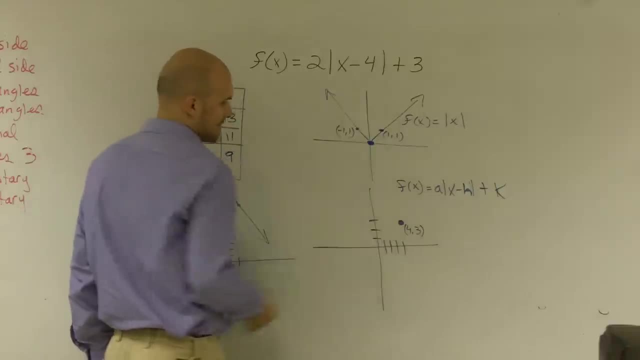 Then now I can pick a point to the left and a point to the right. So now I'll pick. well, we already did negative 1,, right, But let's see. what you guys notice is I picked negative 1,, 0, and 1.. 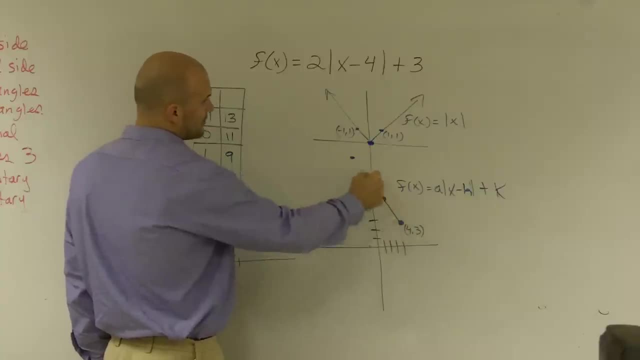 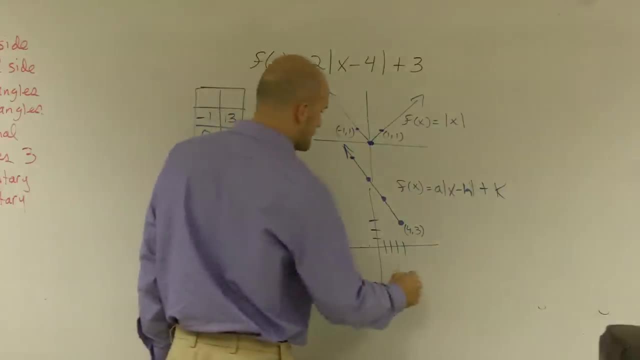 So let's pick 5.. So I'll do: f of 5 equals 2 times x minus 5,, or 5 minus 4, plus 3.. Well, 5 minus 4 is 1.. Absolute value of 1 is 1.. 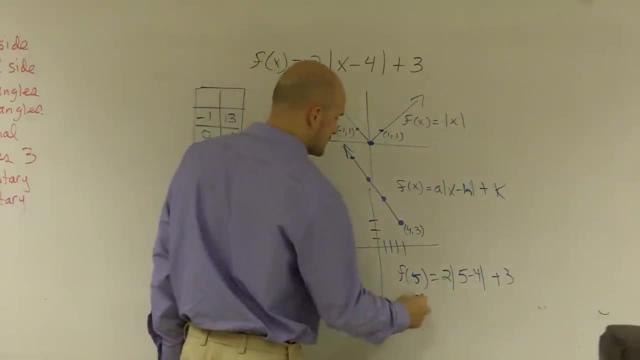 1 times 2 is 2.. 2 plus 3 is 5.. So f of 5 equals 5.. So let's go over here, Let's go over 5 and then go up 5.. 1,, 2,, 3, and there you go. 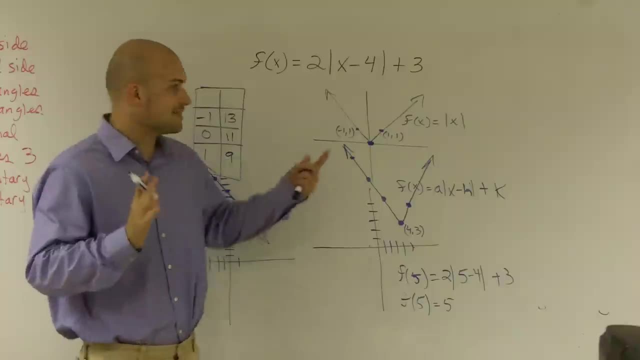 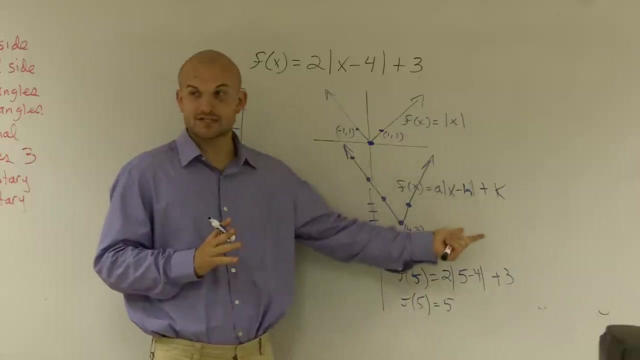 You guys see how that works. So whenever you're graphing absolute value function, especially whenever you see a shift left or right, make sure you find the vertex first by using your transformations and then plugging points to the left and a point to the right of the vertex.